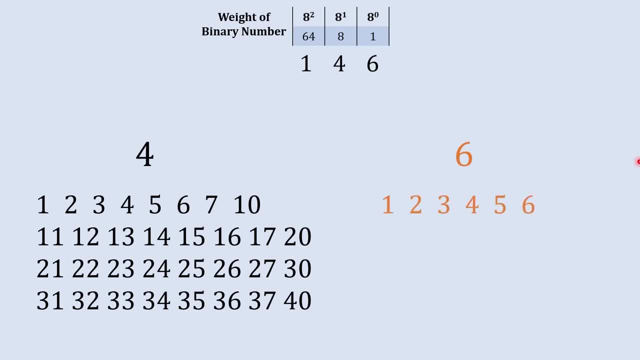 can have six sets of ones, which makes it six, and together this becomes forty plus six, forty six, on which we are focusing right now. Now we want to subtract the 067 from this 146. so here, if we start with the first set, the point of which we can subtract, the point of where the point of difference is, Now, let's count it, Let's subtract it, This is 067 from this 146.. So here, if we start with the 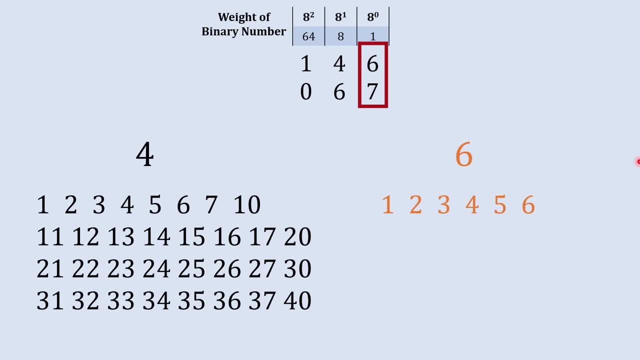 letter. this 7 cannot be subtracted from 6.. So what do we do? We ask for 1, borrow from the next column, and the next column is 8's place. So what do we do? Here we have a 4 sets of 8. So we give. 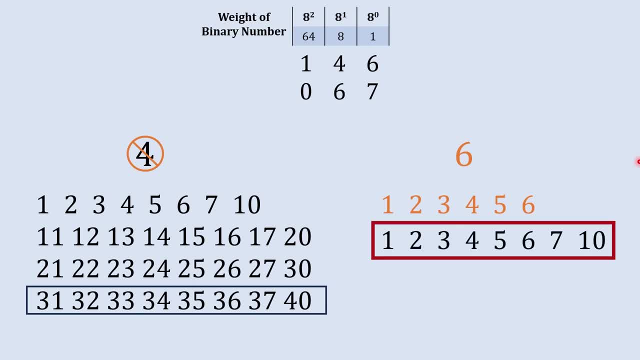 1 set of 8 to the next column, and when we give 1 set of 8, what's left behind is 4 minus 1 is equal to 3.. So now we have 30 here. Now, here this column is 1's column, So we have to consider: 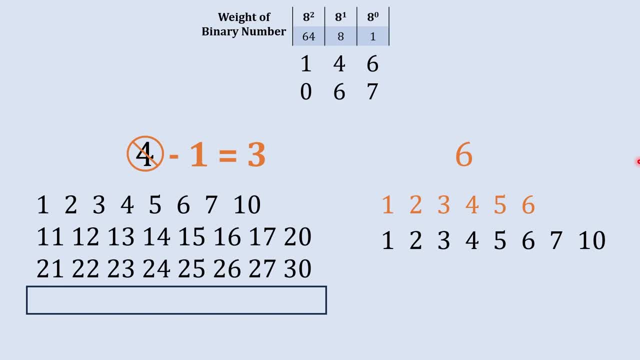 sets of 1's. So how many sets of 1's we have here? Previously we have 6 sets of 1's, and then we have added 8 sets of 1's, So total it becomes 8 plus 6 is 14.. So now we have 14 over here, and 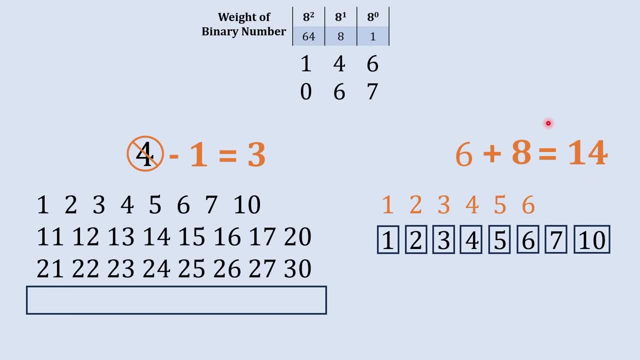 we are going to subtract this 7 from this 14.. So after understanding this logic, now let's get back to our subtraction. But before that, if you are enjoying this video and want to appreciate my work, hit the like button and for more similar. 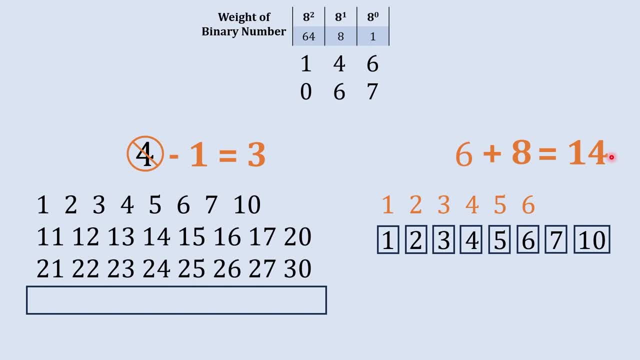 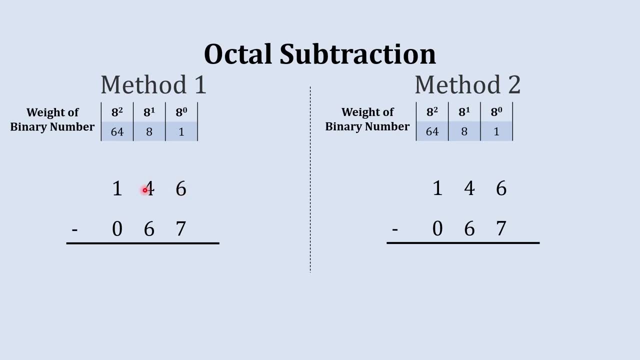 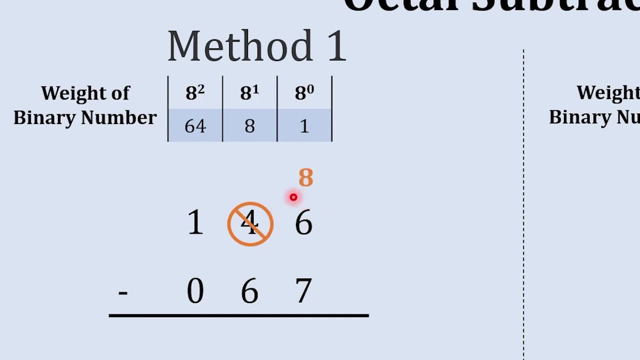 content subscribe to this channel. So done with that. now let's get back to our octal subtraction. So in order to subtract this 7 from this 6, we'll ask for the borrow from the next column. So this 4 gives borrow to this column, So it becomes 8 over here and when it gives borrow. 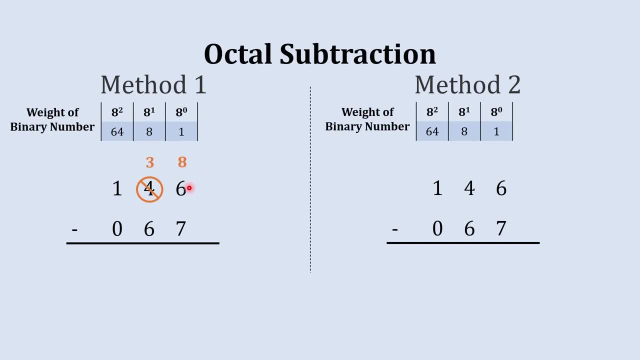 what's left 8 over here it's 3.. So now 8 plus 6 is 14. and now subtract this 7 from 14, we'll get 7.. Now let's see in method 2, when you try to subtract this 7 from 6, it's not possible. So again, we'll go for. 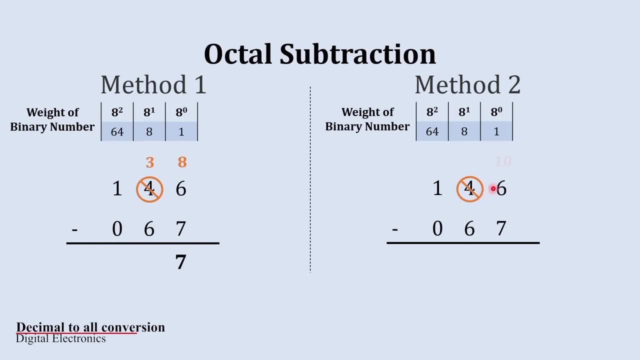 borrow. So this 4 gives borrow over here. So we'll get 1: 0 over here. But how 1 0?? Because in octal number there is no 8, but the equivalent to 8 is 1: 0.. So that is why we write. 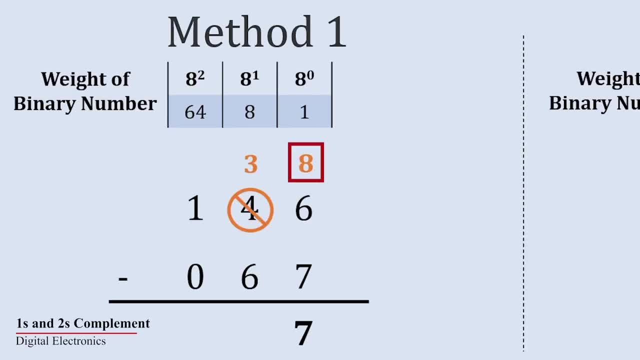 1, 0 over here In method 1, we have used 8 and we have added 8 with 16 and we got 14.. But remember this: here we consider it as decimal numbers and we do addition and subtraction of these numbers as 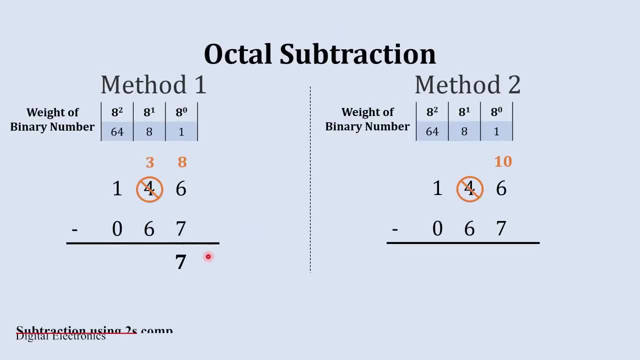 decimal numbers, But the end result we'll get will be always octal. So now let's come back to method 2.. Here we have 10 and 6, and when we add them together we get 1- 6 in octal. 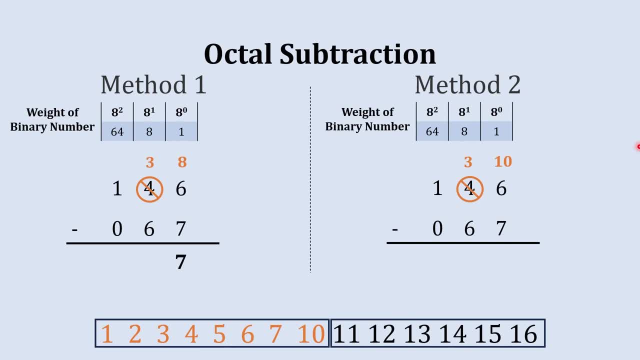 Here we'll use real octal numbers. So after 7, it's 1, 0, and so on. It's not 8,, 9,, 10.. After 7, it's directly 1, 0.. Now let's get back to subtraction again. So 10 plus 6 is 16.. That is. 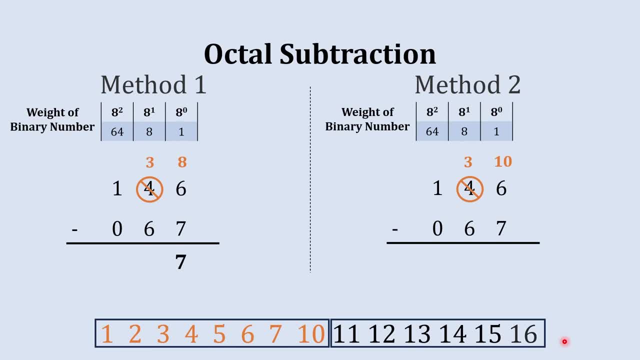 what we get here. So now let's subtract this: 7 from 16.. 1,, 2,, 3,, 4,, 5,, 6 and 7.. So when we subtract 7 from 16, we get 7.. So when we subtract 7 from 16 octal, we get. 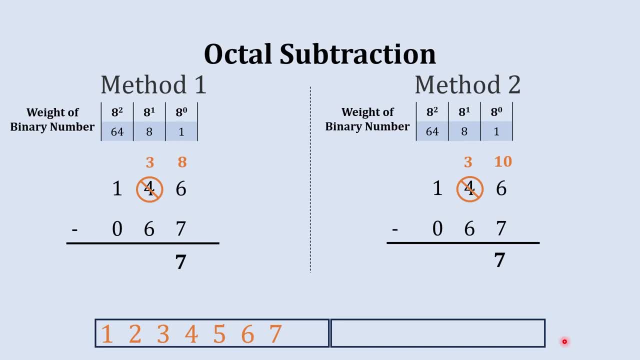 7.. So that's how we do subtraction in method 2.. Now we'll jump to the next column. Here we are going to subtract this 6 from this 3, but it is not possible. So what do we do? We'll again ask for. 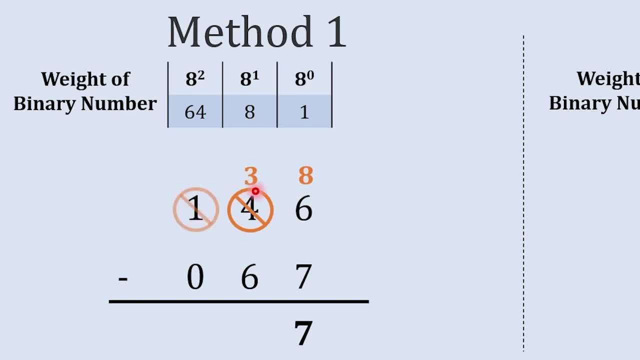 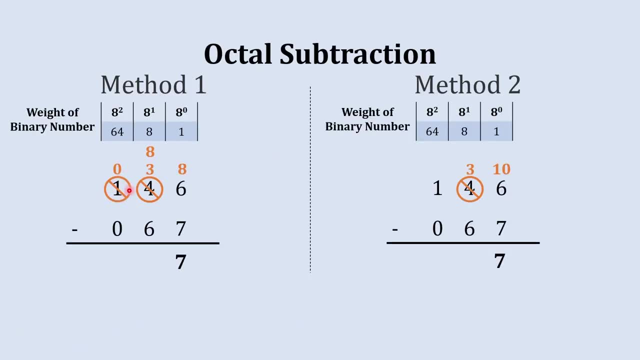 borrow from the next column. So when this 1 gives borrow to this column, it's 8 over here and what's left over here It's 0, because here there was only 1 and we have given this 1 as borrow to the. 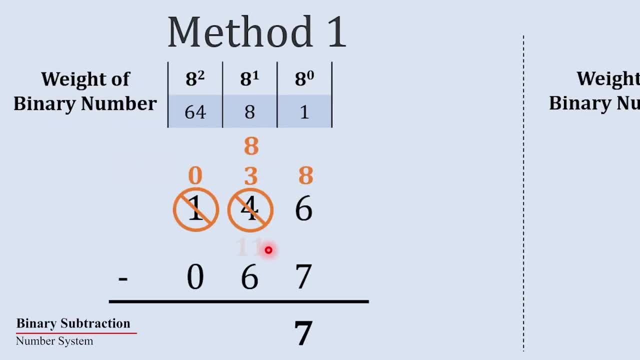 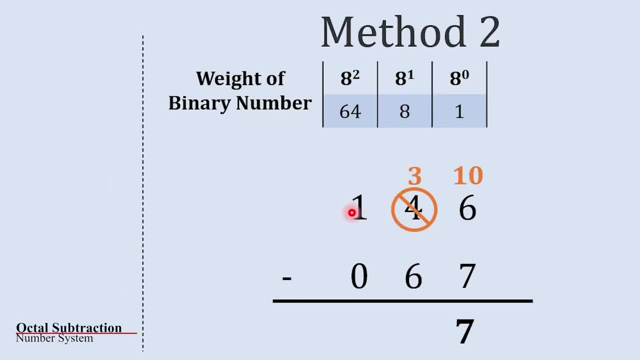 previous column. So we're left with 0 over here. So now this 8 plus 3 is 11 and 11 minus 6 is 5.. Now we'll do the same process in method number 2.. So when this 1 gives borrow to this column. 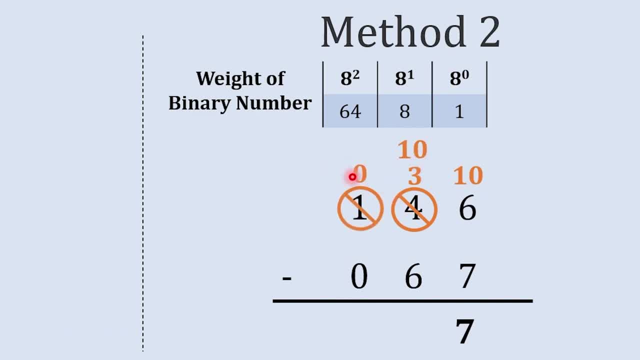 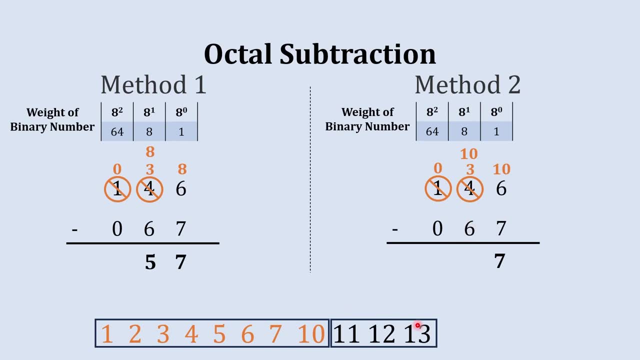 it becomes 1, 0 and 0 left over here. So here we have 1, 0 and 3.. It's 13 in octal, So we are going to subtract this 6 from this 13.. So let's subtract 6 from this 13 and we're left with 5.. So 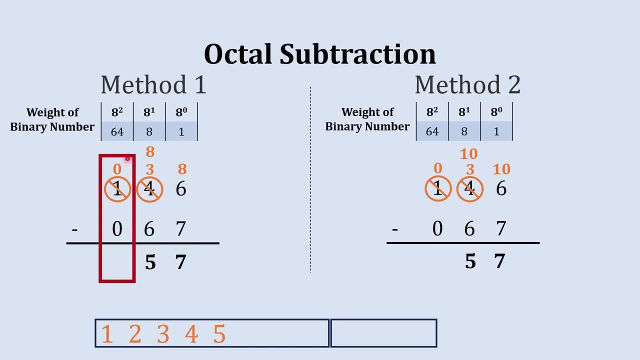 5 will come over here. and now let's see the final column: 0 minus 0 gives us 0.. The same way, 0 minus 0 gives us 0. So finally, the octal subtraction is 5, 7.. This was little bit simple. Now I'll. 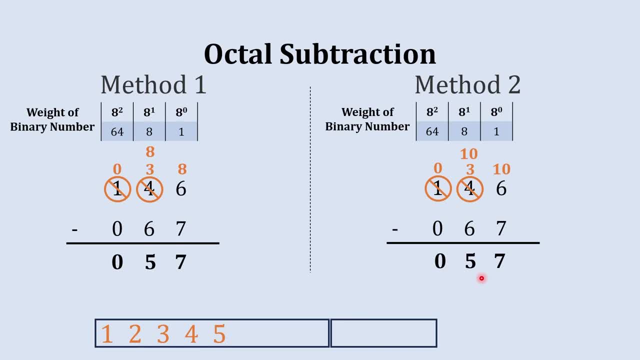 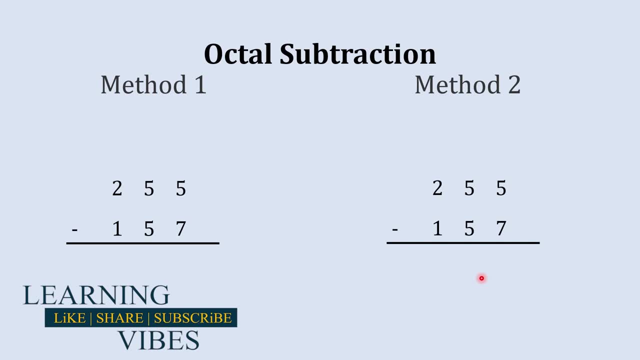 show you little bit more complex octal subtraction than this one. So let's jump to that. So here we have these two numbers and the same way we have two methods to solve this. So here we'll start with the left most column. We'll subtract the 7 from 5, but it is not possible, So this 5. 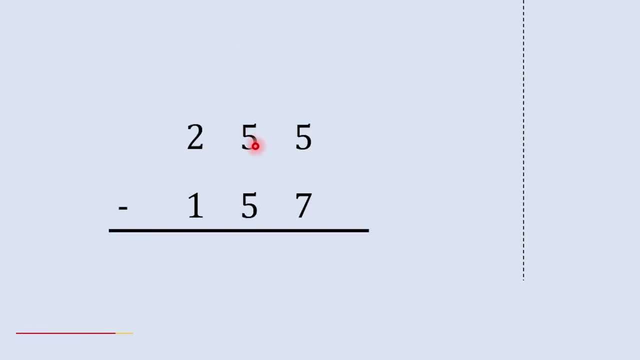 will ask for borrow from the next column. So when this 5 gives borrow to this column, it's 8 over here and what's left over here? 5 minus 1, that is 4.. So now here, 8 plus 5 is 13.. So 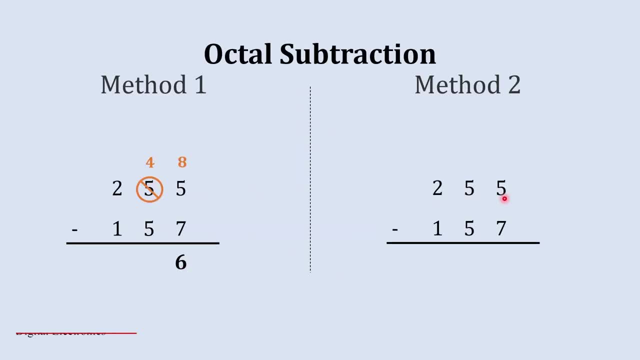 13 minus 7 gives us 6.. If we do it in method number 2, this 5 will ask for a borrow with this 5.. When this gives borrow, it's 1, 0 over here and 4 over here. So 1, 0 plus 5 is 1, 5 in octal. 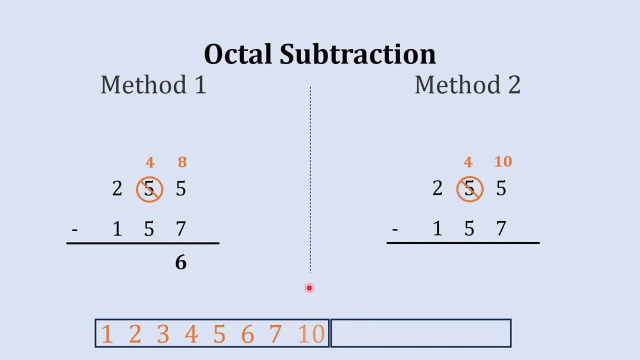 So when we subtract 7 from this 1,, 5, what do we get? We get 6.. So we'll write 6 over here and we'll jump for the next column. So we are trying to subtract this 5 from this 4, but it is not. 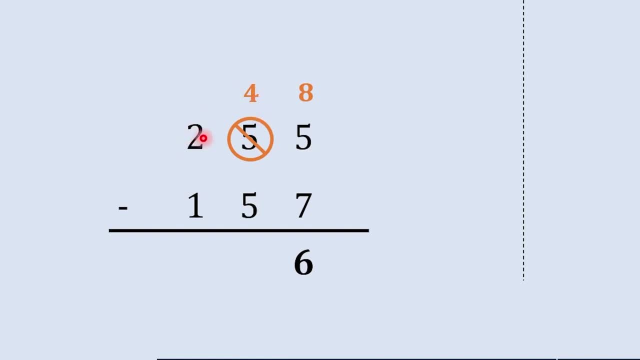 possible. So what do we do? We again ask for a borrow from the next column. So when this 2 gives borrow, it's 8 over here and 1 will be left over here. So 8 plus 4 is 12, and now we subtract this. 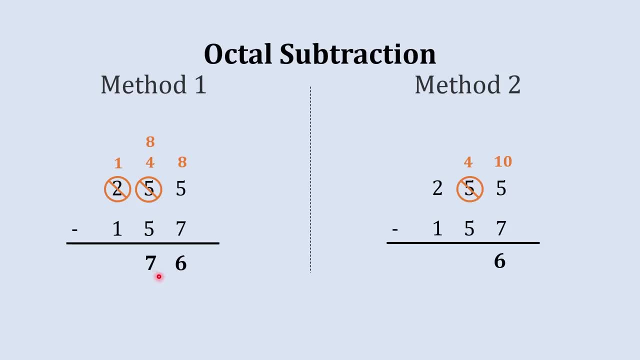 5 from this 12 and we get 7.. If we do the same process in method number 2, this 2 will give borrow over here and it's 1, 0 over here and it's 1 over here. So 1, 0 plus 4 is 14 in octal. So when we subtract this 5 from this 14, what we are going 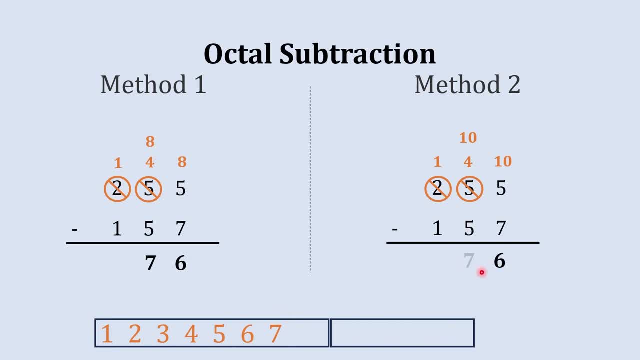 to get. We are going to get 7.. So we'll write that 7 over here. and then finally, the last column: 1 minus 1 is 0.. Over here also, 1 minus 1 is 0.. So the final octal subtraction is 7, 6 and then 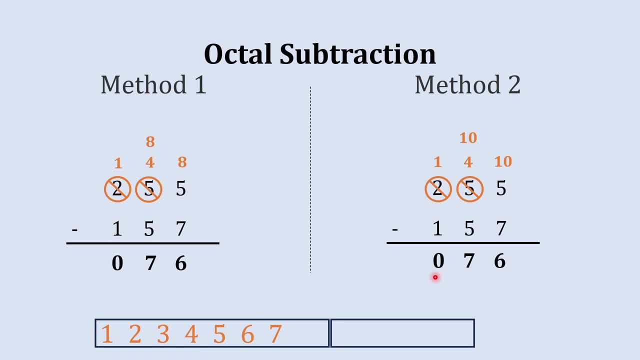 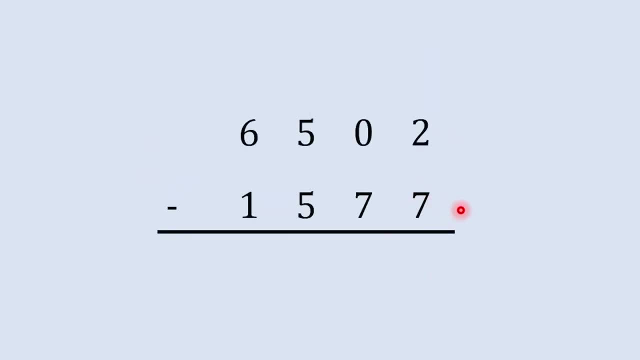 finally, I'm going to show you the most complex subtraction out of all these three, with the octal. So now let's jump to that. Here we have these two octal numbers and we are going to subtract these two. So first of all, we'll try to subtract 7 from 2. It is not possible. So this 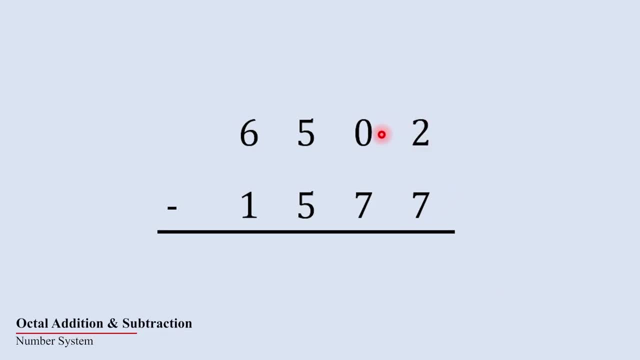 2 will ask for a borrow to the next column. but see over here, this next column is 0. So itself, this column is incapable of giving borrow. So what do we do now? So now, first of all this: 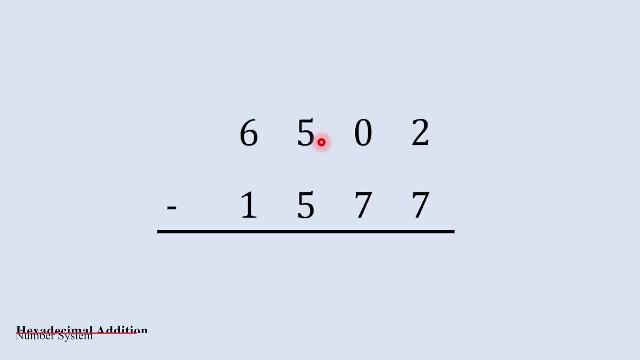 column will ask for a borrow to this column and check if this column is capable enough. Yes, it can give borrow. So now let's jump to that. So let's jump to that. So now let's jump to that. So. 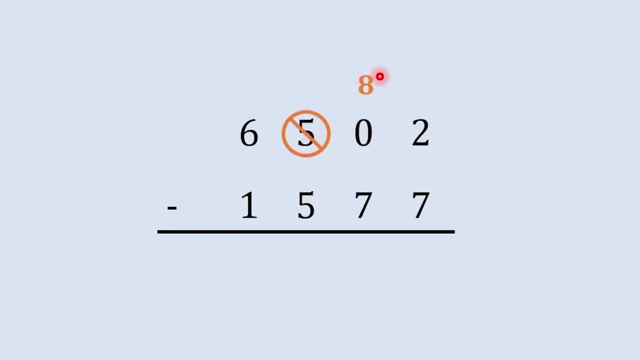 now this 5 gives borrow over here, So it's 8 over here and 4 will be left over here. So now in this column we have 8.. So now this column is capable enough to give borrow to the previous. 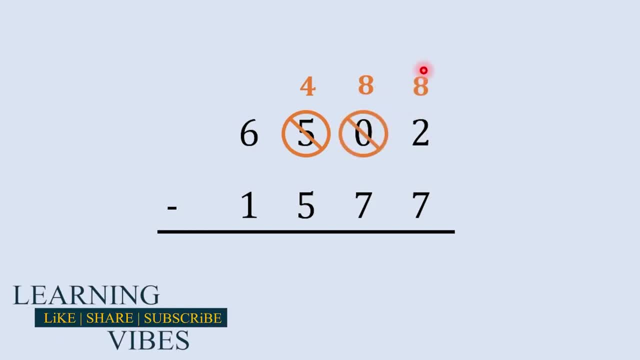 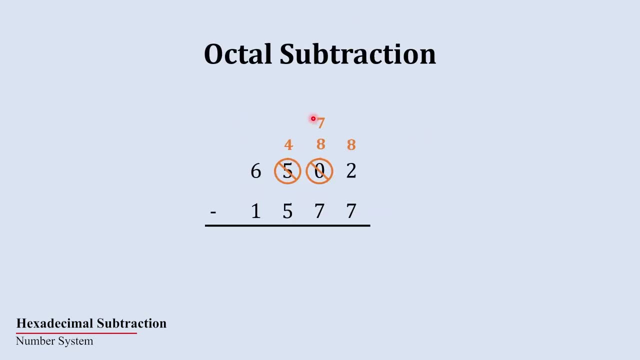 column. So when this column gives borrow to the previous one, it's 8 over here and what's left over here? Previously it was 8. So now it will be 7 only, and now we'll do subtraction, So here. 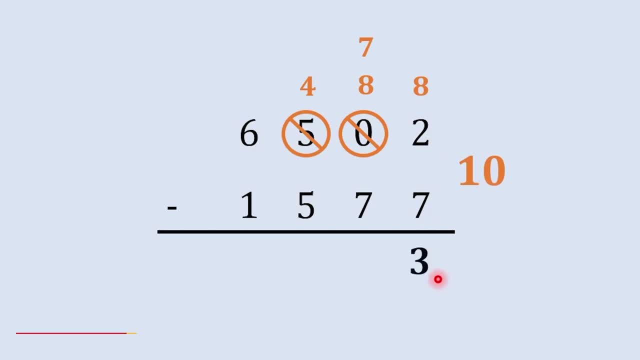 8 plus 2 is 10.. So 10 minus 7 is 3, and then we'll jump for the next column. Here we have 7, and what's left here? previously It was also 7.. So 7 minus 7, we get 0 over here, and then we'll jump for the next column. Here we have 5. 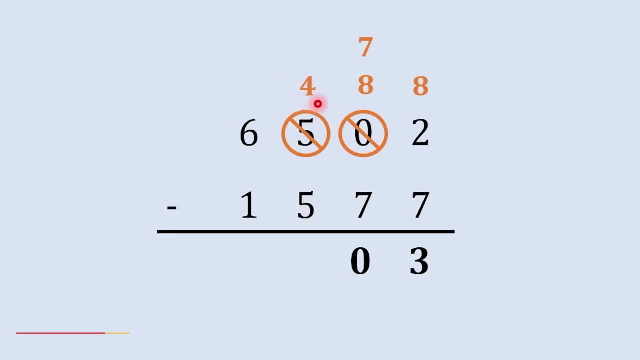 and we are going to subtract this 5 from this 4, but it is not possible. So, again, this will ask for the borrow from the next column. So this 6 will give borrow to this column. So it will be. 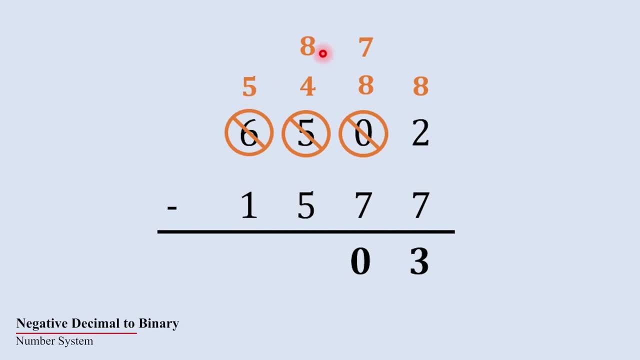 8 over here and 5 will be left over here. So now here, 8 plus 4 is 12.. So 12 minus this 5, we get 7, and then we'll jump to the next column. So here we have 1.. Here we have 5.. So 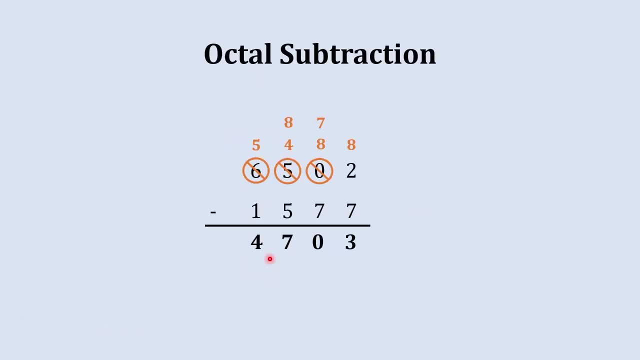 1 minus 5, we get 4.. So final octal subtraction is 4703 and that's how you can do the octal subtraction Here. I have shared two examples for your self-practice. Do it now and write the. 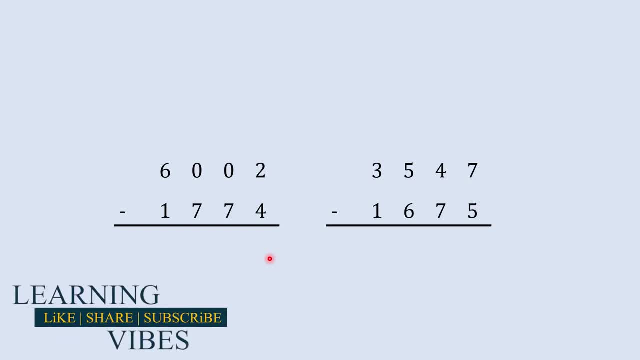 answer in comments to check the answer you got is correct or not. Like this: if you want to learn multiplication, then click on this video, and for other octal arithmetic operations or binary arithmetic operations, you can refer these playlists. So see you into the next video of. octal multiplication.